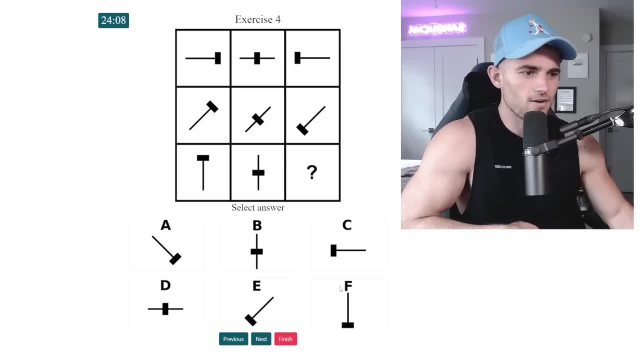 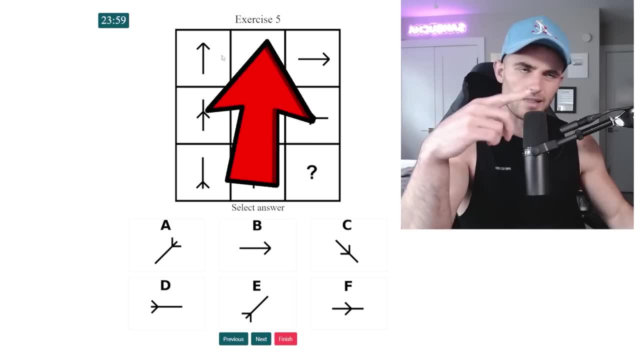 right center, left, right, center, left, up, down. So it's going to be down and vertical. So F Feeling good. so far, All right. This is more of the same, So it looks like it's going clockwise. 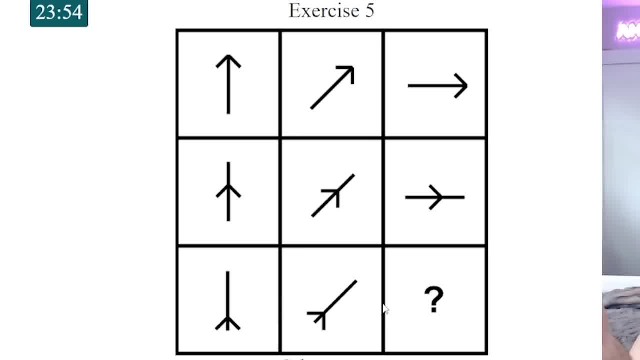 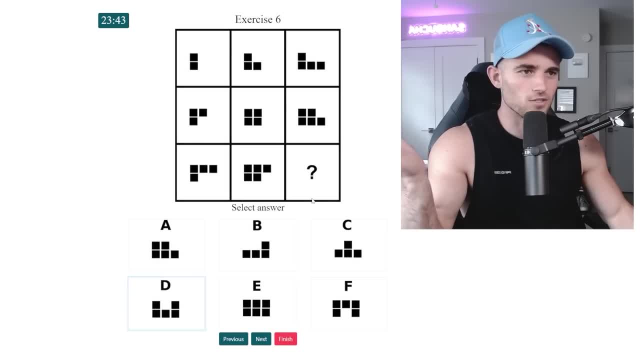 Everything's going clockwise, Great, And the tail just moves towards the bottom. So it's going to be E right? Does that sound right? Okay, I want to make sure I don't want to get like easy questions wrong. All right, Block. 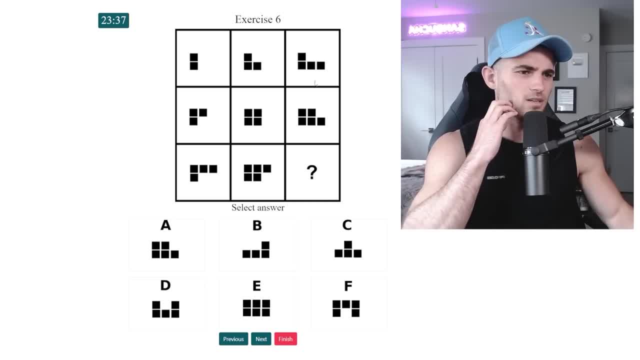 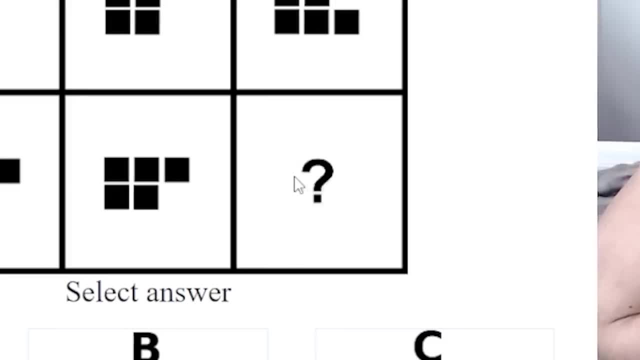 block, block. Okay, I think I'm seeing what's happening here. Hold on. They were just adding: So three four five, two, three, four, four five. There's going to be six And it looks like. 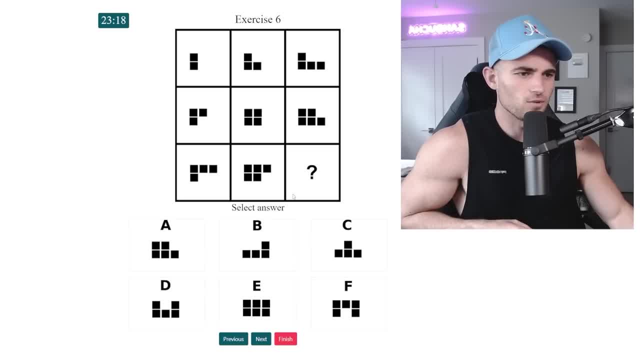 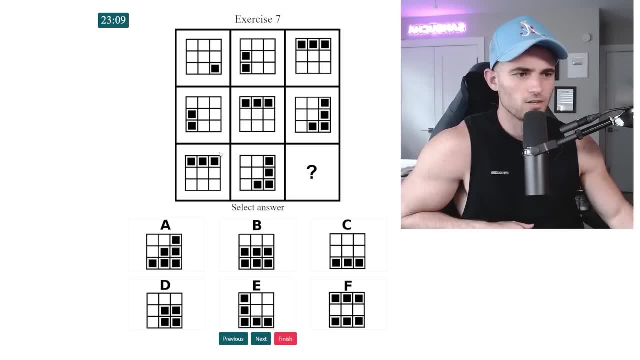 it's going to be. it's all additive, So it would make sense that it's E right, That's the only one with six, anyways, Okay, One, two, three, two, three, four, three, four, five. So there's going. 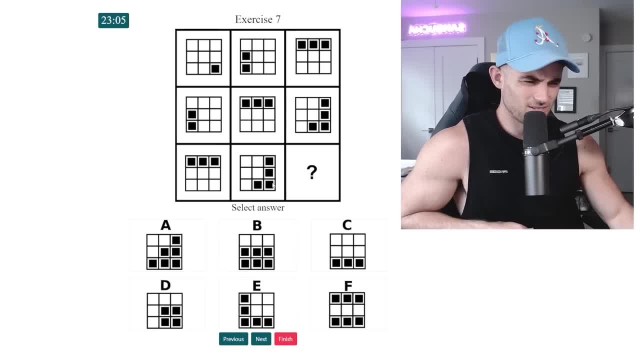 to be five, and it's kind of snaking around. So I would say M, then two, then three. All right, So they're filling out this first. So it's going to be three on the bottom, followed by two up top. So where's that? Yep, Three on the bottom, two up. 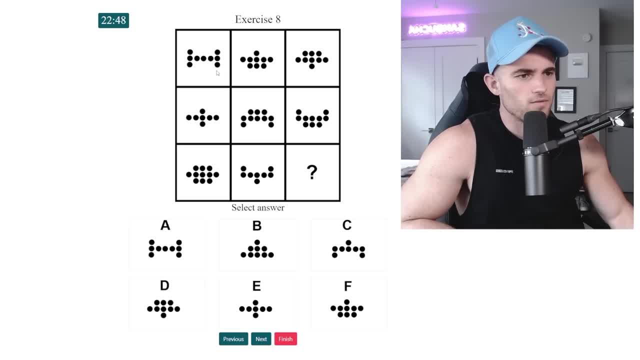 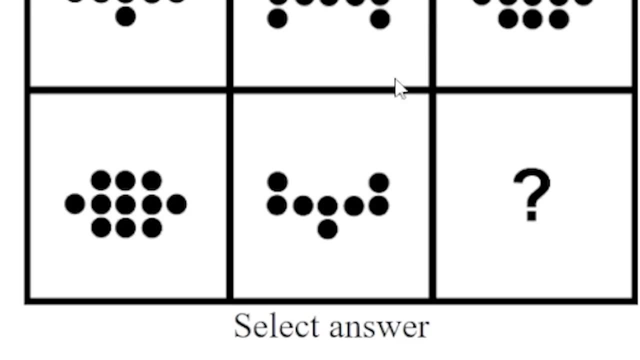 top. So E, All right, We have, what do we have here? An H, and then that flips, that flips. So this is going to be this flip. So this is kind of like a decoy one, I'm guessing. So the idea is to 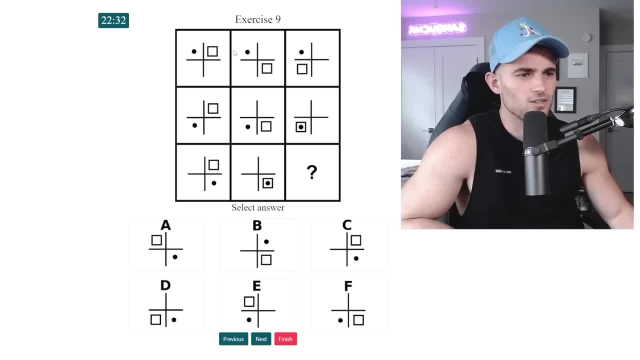 have this as C, I'm pretty sure. All right. So we have the dot doesn't move, So it's going to be a bottom right dot, So it's going to be A or D And then in terms of this, so if we just look vertically, it's top right. 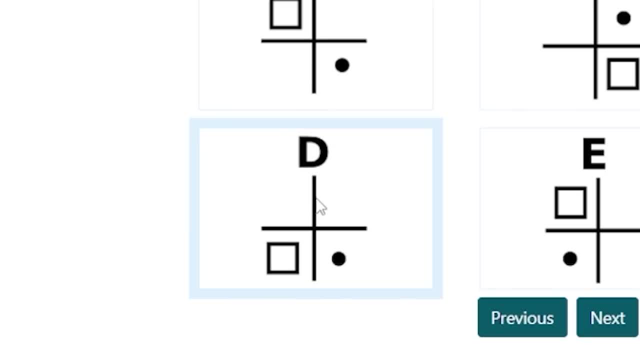 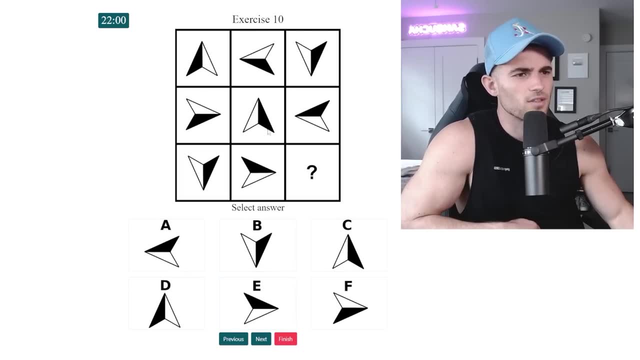 bottom right, there's going to be bottom left, So it's got to be D. Right side, this is going to be. the left side is going to be highlighted, which brings it to either D or E. And then what direction are things looking like? Bam, bam, It's going to be up, So it's going to be D. I felt the least. 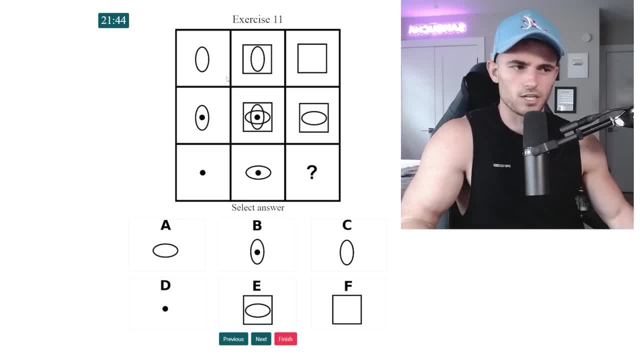 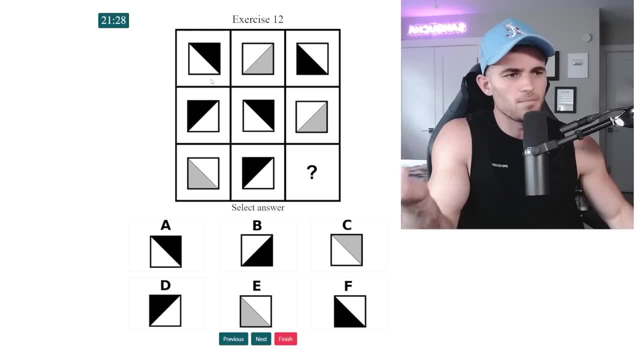 confident about that one. All right, so it looks like subtraction. Does that sound right? So we have this minus. this equals this, this minus, this equals this, this minus. this equals A: Top right, bottom right, bottom left, top left, top right, bottom right. 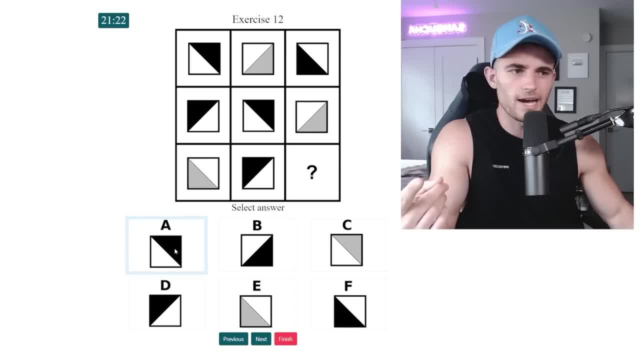 So it's going to be Dun dun dun. So it's going to be top right, and I'm guessing it's going to be black, because there's only one gray scale in each of the rows. So A there's going to be a triangle. that's the missing shape, And 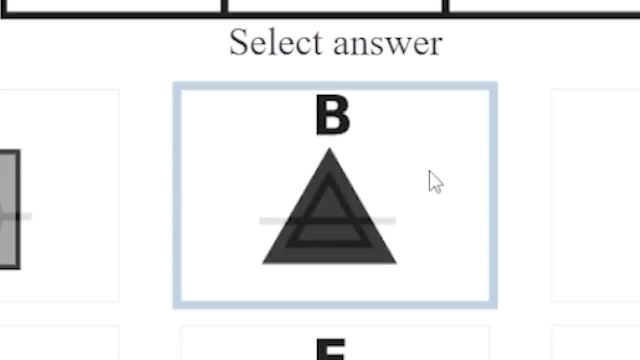 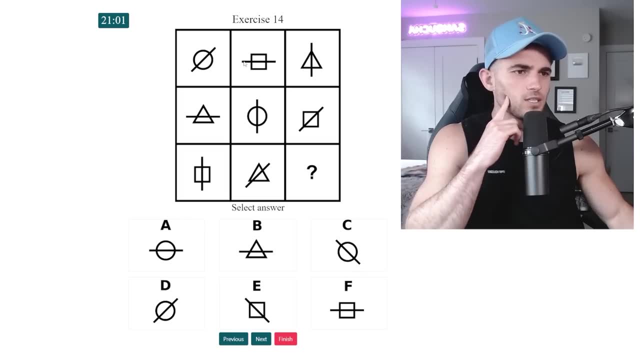 it's going to be a black triangle. that makes the most sense, right? black triangle. Final answer: be All right. So once again, the missing shape circle. and now which way is the line going to be? good question, sam. the answer to that is: 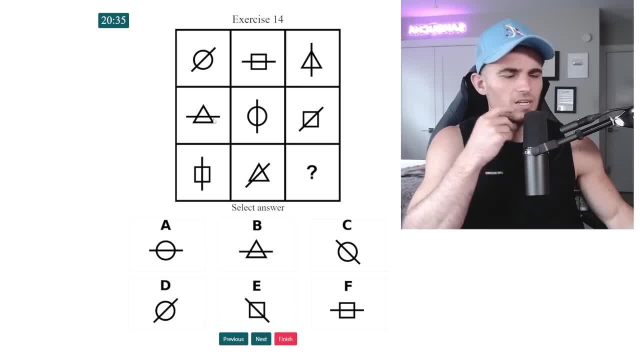 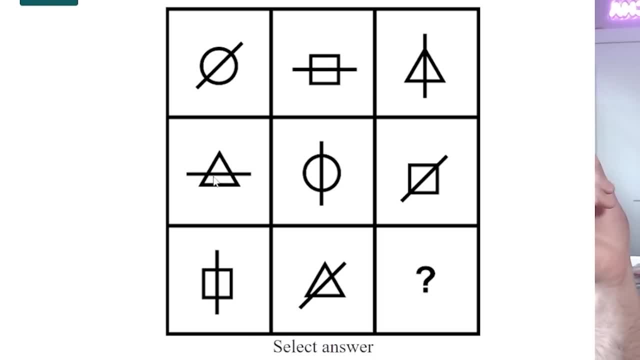 um, there's not really like a theme to the way that the line falls. okay, i see it's going to be a horizontal line through, because that's there's a horizontal line and everyone but this. so it's going to be circle with horizontal line. i don't know why that took me so long. one, three, two, three. 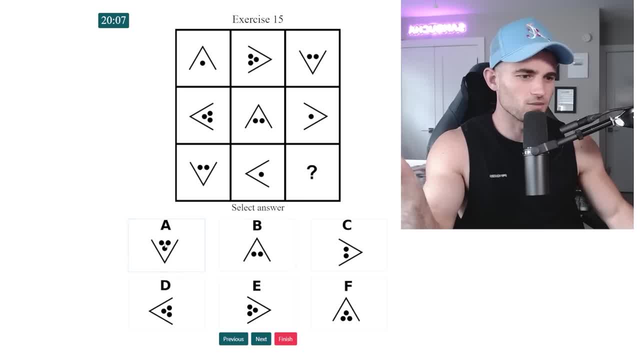 two, one, there's going to be three in it, and then so again direction. so which direction? so it's going to be a, d, e or f, and then the direction of this is going to be up. so f, okay, all right. so it's going to be a white one, so it's going to be a, b or f, and then, in terms of direction, it's going. 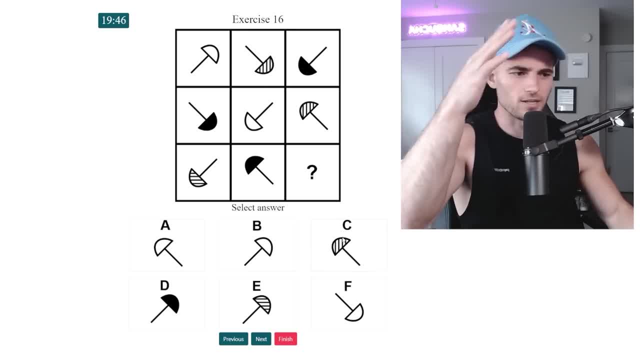 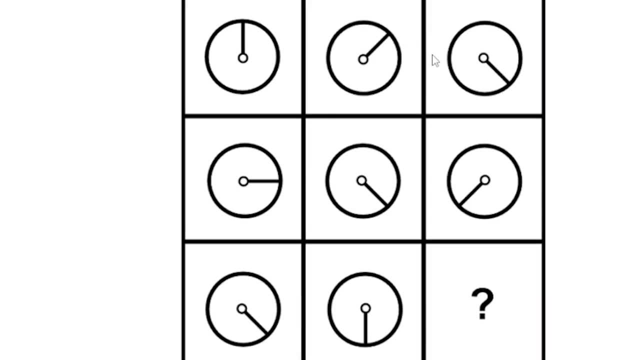 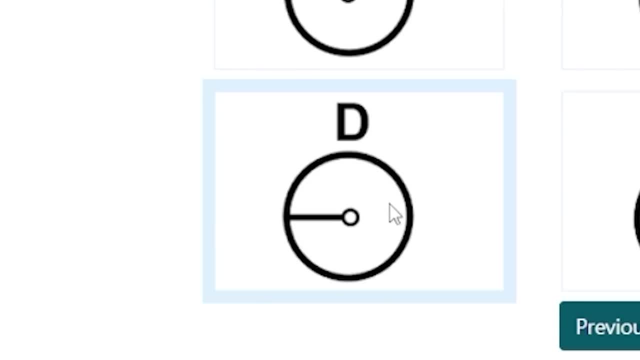 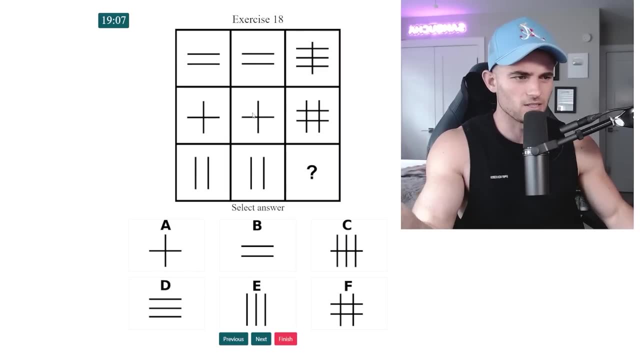 45, 45. that sound right. so it'll be d uh, equals. okay, this is weird. so clearly these are all uniform and they mean something. so let's see total intersections, for instance: one, two, three, four. one, two, three, four, eight. one, two, three, four, five, six, seven, eight, nine. okay, that's not it. 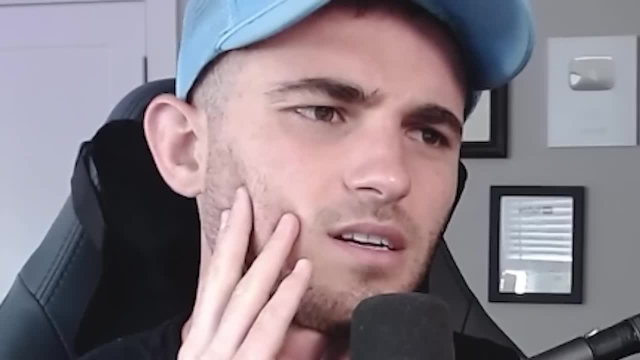 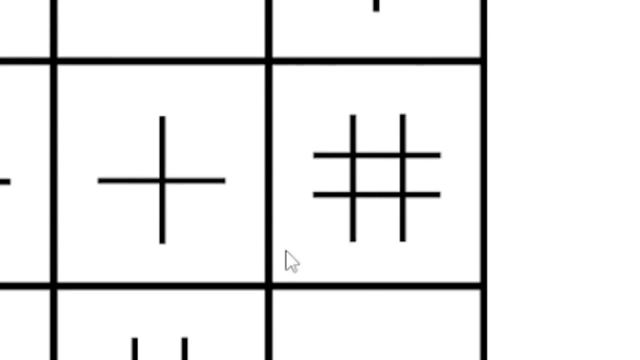 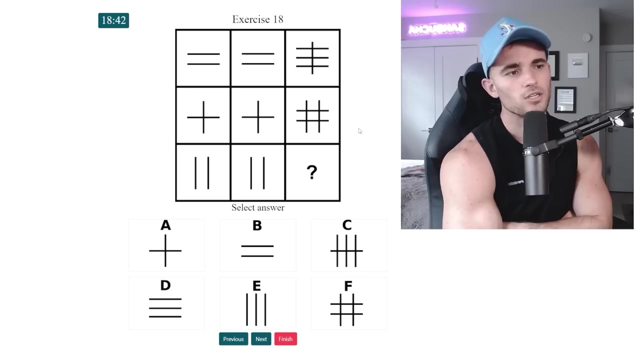 um, all right, what we can. what do we learn from this? okay, the total line. so there's four lines: one, two, three, four. one, two, three, four. i guess they're all four lines, but the way in which they interact with each other is interesting, isn't it? so i think the best guess is that it would be the 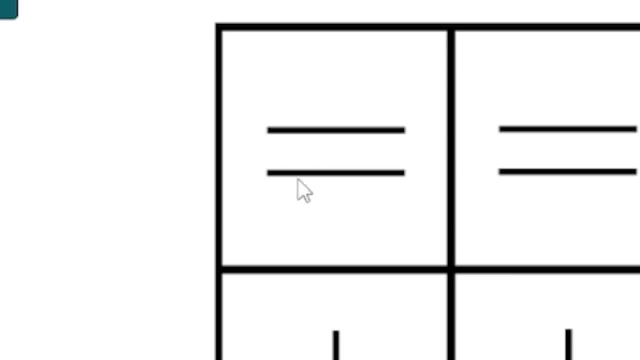 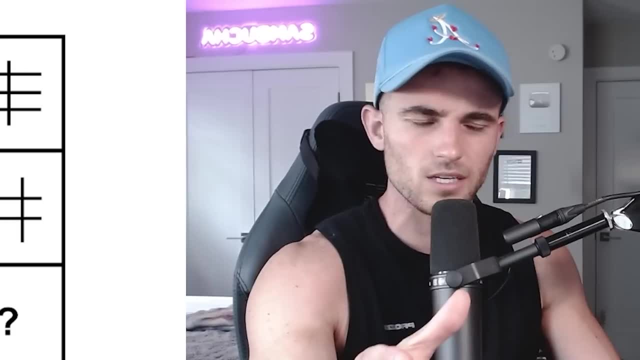 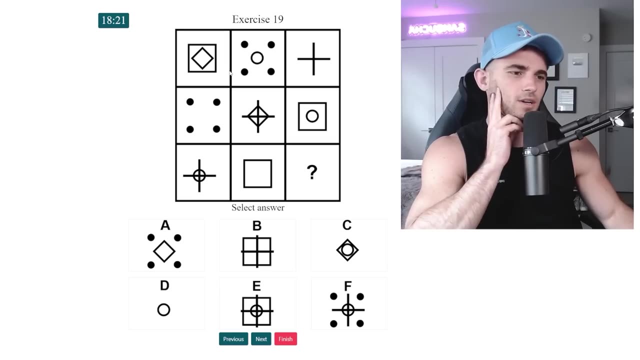 inverse of this, because these two verticals are essentially, yeah, the vertical version of up here, so we effectively will just have to turn that, in which case it would be c. does that make sense? it does to me. so we're doing it all right now. uh, okay, i think i know what's going on here. i think 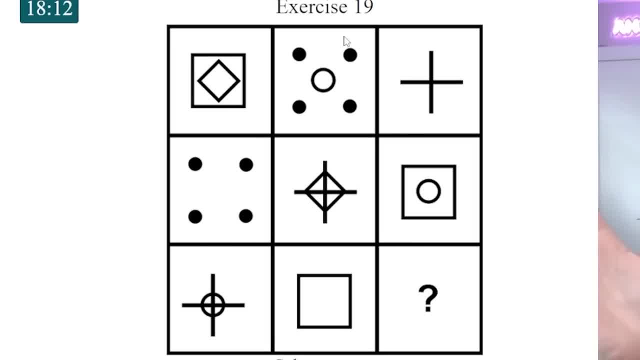 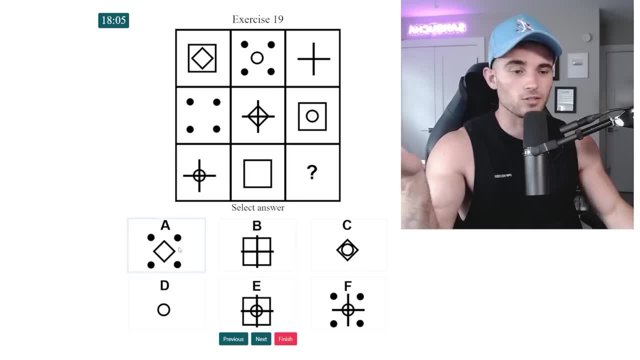 we need to have all of these elements that are present here down here. so we don't have four dots, for instance, so we need four dots, so it's going to be a or f off the off the rip. we don't have a triangle, so it's. 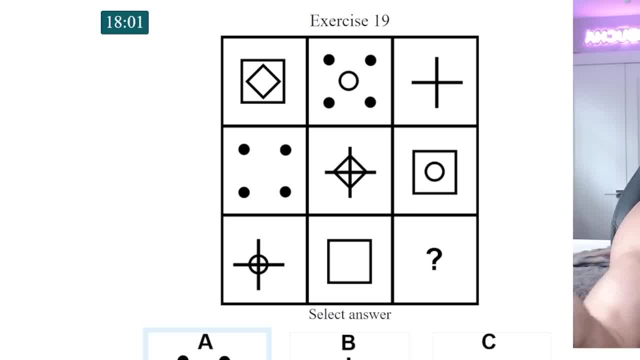 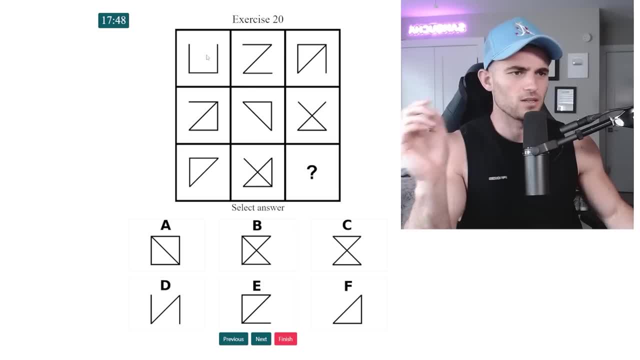 got to be a, so it's not going to be f. it's got to be a because we're missing the triangle in the four dots: u z, bam, bam. okay, so what it looks like is a combination, but if there's overlap it eliminates it. so it's this plus this, minus the shared variable, which in this case would be say: 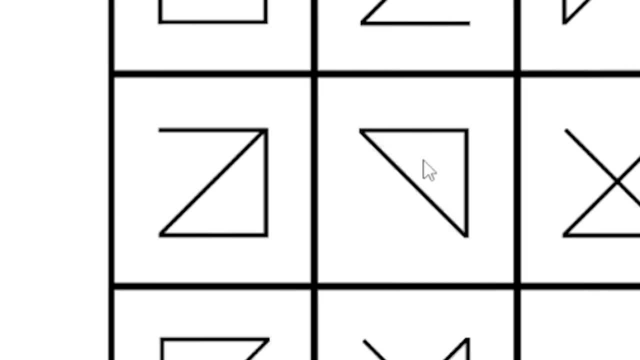 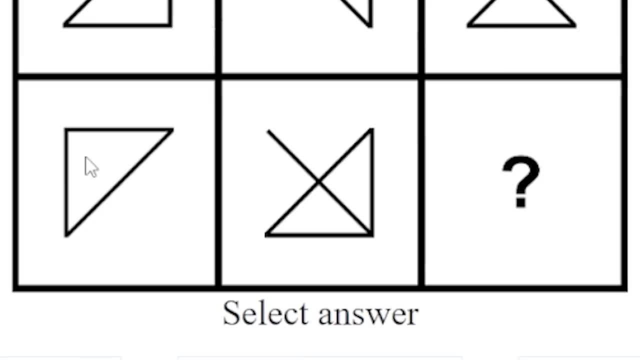 the bottom line. let's see, the bottom line disappears. so we're going to have a combination. appears this plus this same sort of story: there's a common line of the top and side, therefore it's eliminated. so then this: what is the shared line? the shared line is the middle, so there's going to 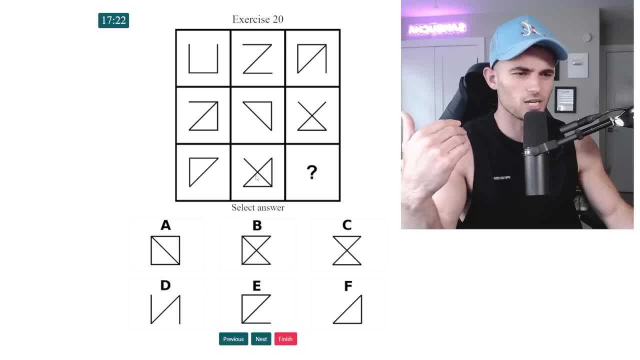 be no line in the middle, like this line right here, because that's the shared line. so now i'm just trying to picture what that would look like. this is a very difficult thing to picture, so i need these two lines. so it's going to be a, b or e, and then what line is getting rid of that middle? 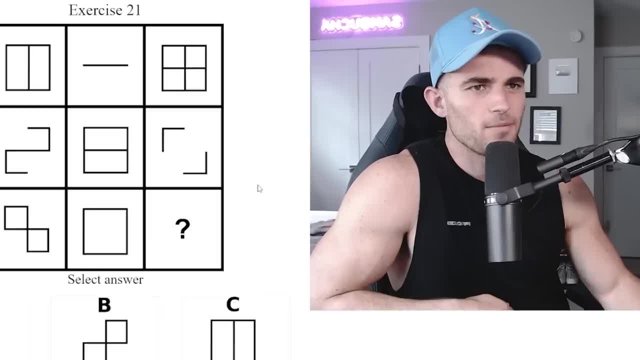 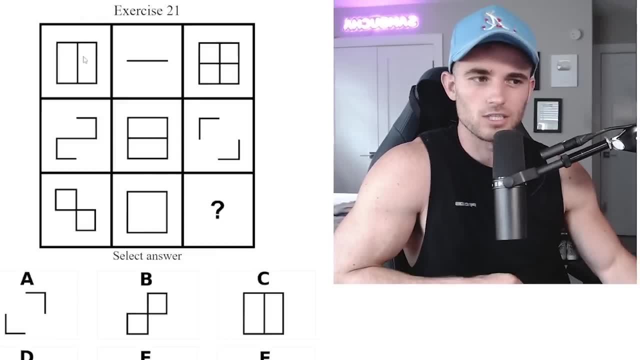 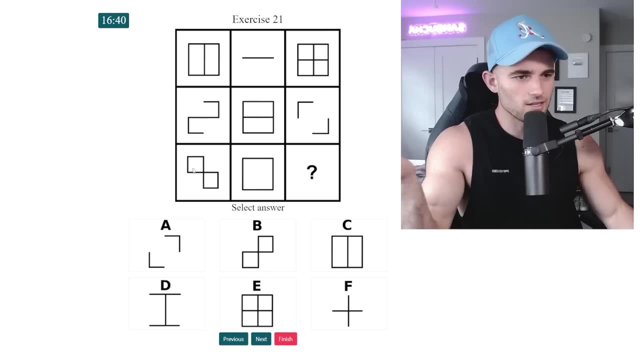 so it's going to be a- i'm pretty positive- 21. how many questions are there? i guess they don't tell me that. um, exercise 21. i'm starting to get like brain rot. all right, this is just additive. looks pretty good, additive, good. um, okay, so it's again. this is additive, and then eliminate the commonality. 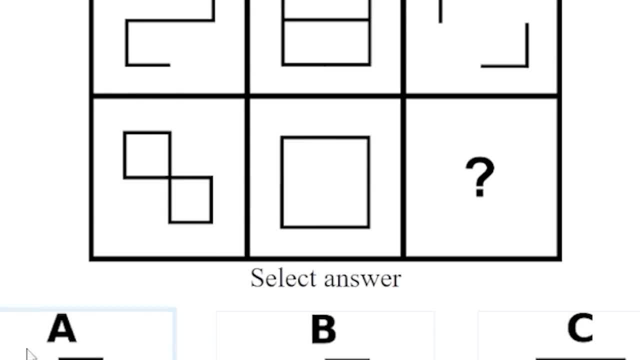 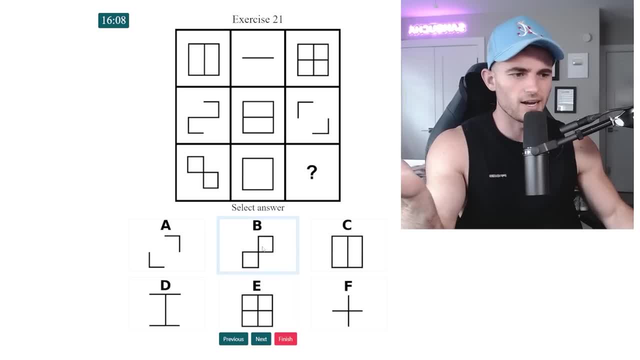 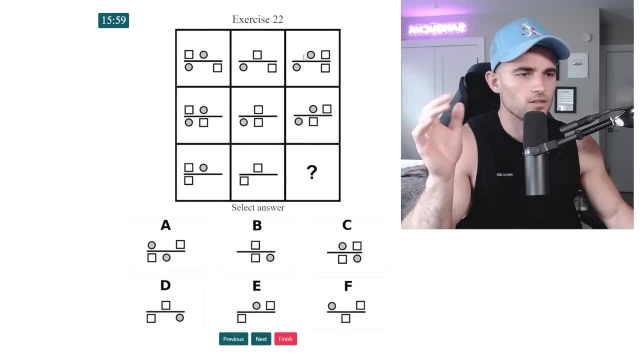 okay, so this is not going to have the top left, so top left disappears, in which case we're only down to a, b or f. yeah, it's got to be b because we're gonna retain the inside lines and there's still going to be a, b or f because there's not overlap. let's say the right top would be square circle. 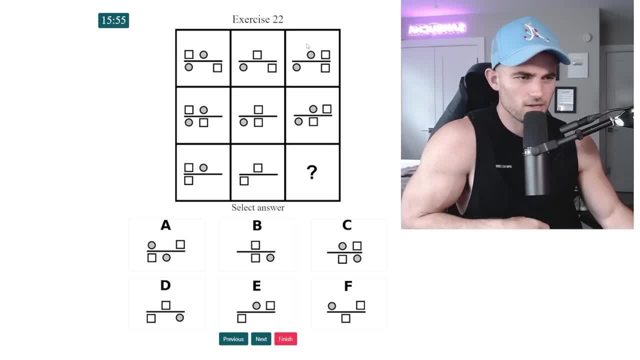 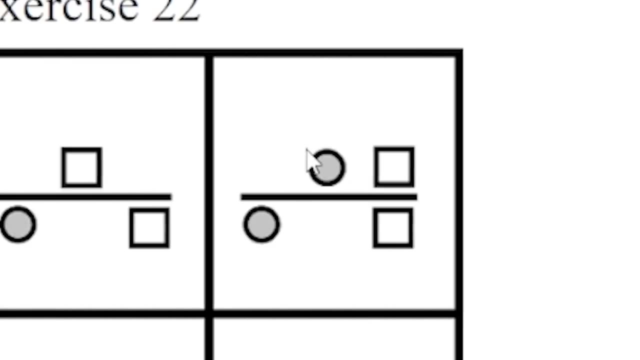 squares. okay, why is this? okay, i see what's happening here. the the square on top is moving one over right in each direction, so it's going to be a top right square. know that? good, the circle is blinking, as i'd say, so it's like middle, nothing middle, or it's only blinking because the square 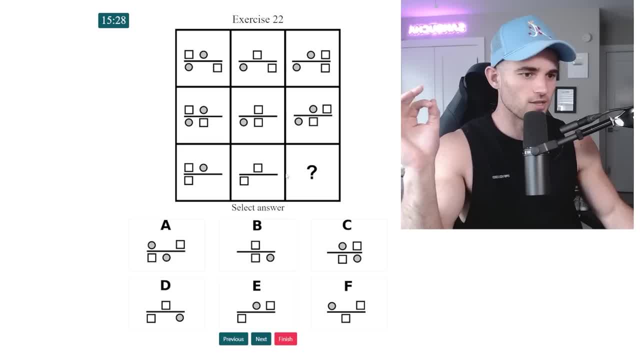 is passing it and you can't have two things, then okay, so i see. so then this is going to return to, uh, the middle, so it's going to look similar to this top right on top. so it's going to be c most likely. let's just make sure everything else checks out. huh, that doesn't make sense, though does 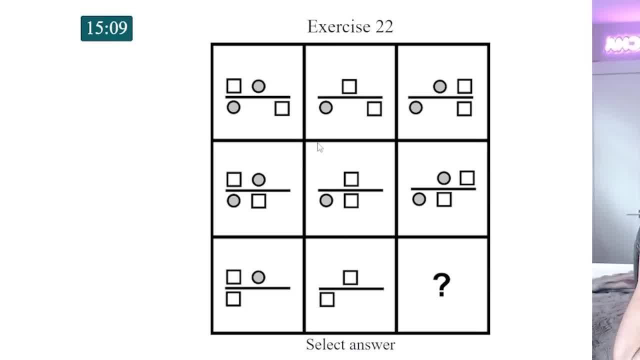 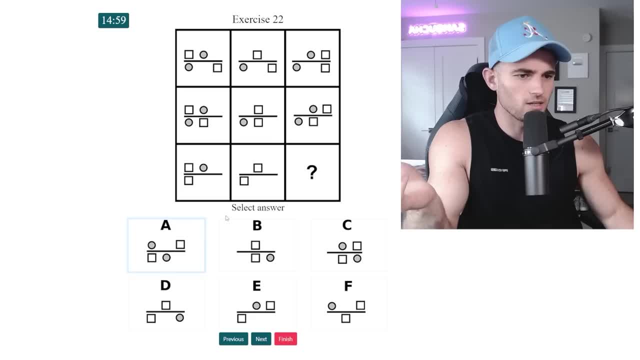 it does, it might. okay, let's just rework this real quick. okay, he moves over, he blinks, he moves over, he blinks, he moves over. so it's going to be to the right. and then he it'd be: oh, sorry, sorry, so it's going to be e. i forgot, i didn't even realize that e is also the same top structure as c, that. 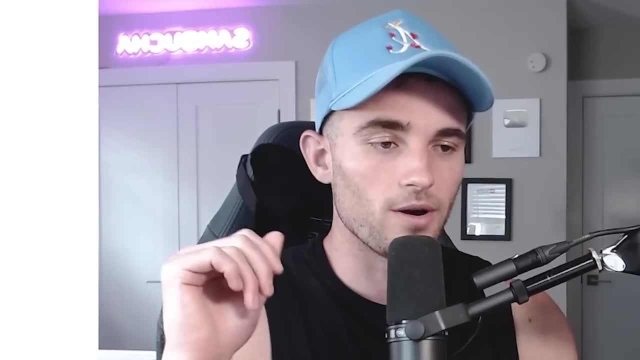 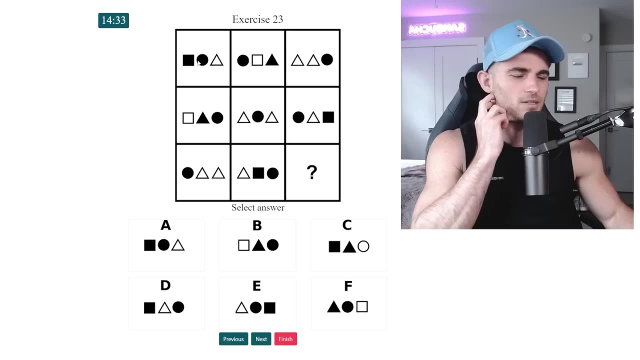 is the same. so yeah, e once again i'm dumb. i'm sorry. what do you want me to do about it? uh, so we have. i am kind of drawing some blanks on this pattern because i don't know what's happening here. looks like there's squares only available in two of them, in which case this is: 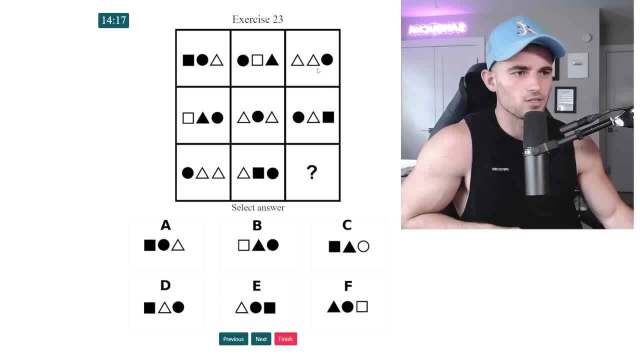 going to have a square on the bottom. we already use our double triangle here, so there's a double triangle in each of them that's used and the circle is always highlighted. there's a square, so we can eliminate the double. there is no double triangles, of course that. 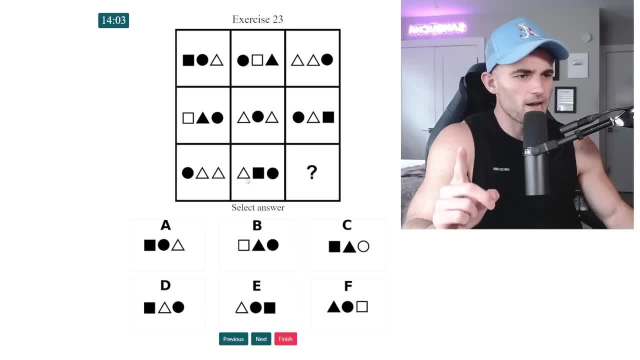 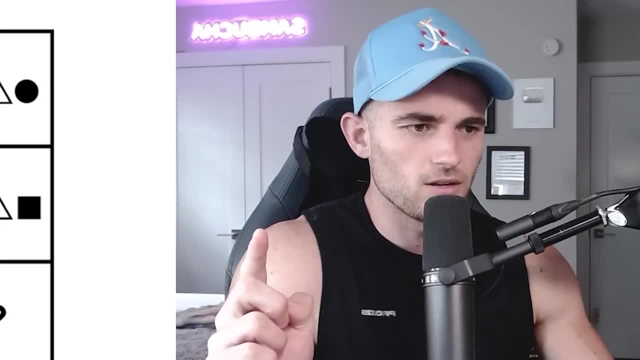 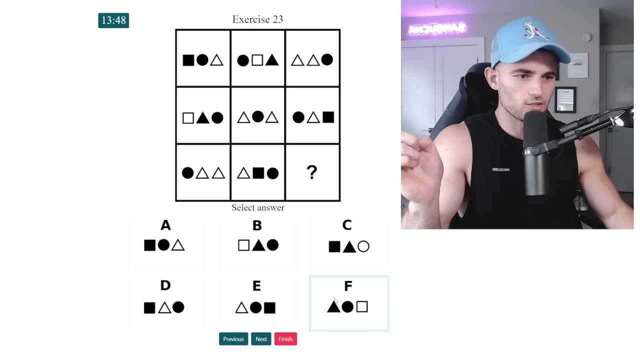 doesn't help us, i guess. um, i'm also curious: is there always a pattern in which it takes on this? there is okay, so there's always going to be a white triangle with two blocks sounded racist, so it's going to be then this structure which is a white square, the white square is. so now we're. 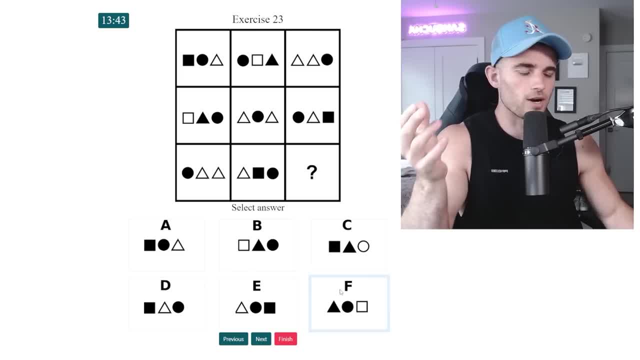 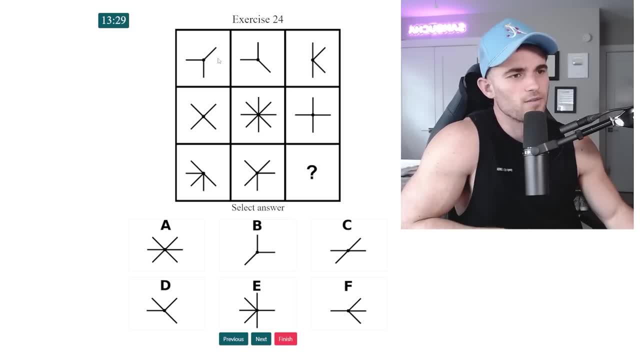 looking at it's b or f. so now i have to figure out the order of the white squares. so the white square is going to be a right middle square, so f, exercise 24. so we have this figure- it's additive- and then once again deleting the commonality, so this left one is then eliminated. okay, so that. 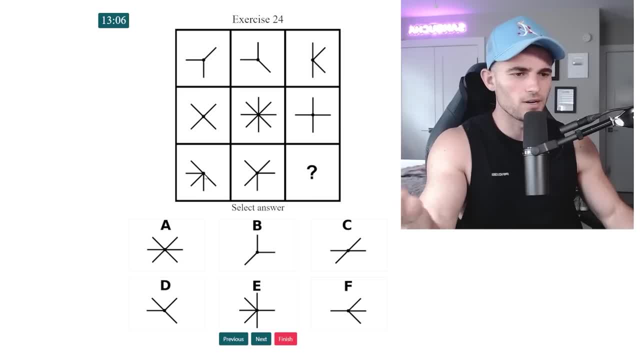 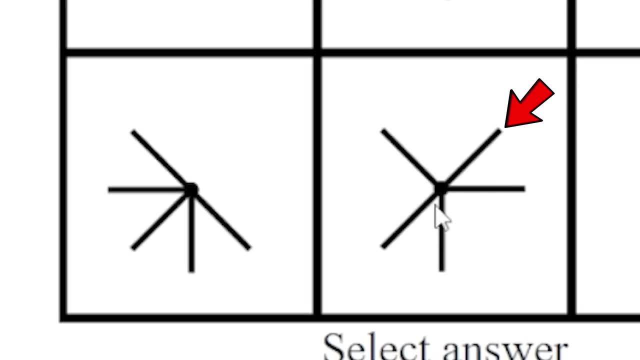 makes it pretty easy. so let's assume i'm not even going to go through the middle one. i'm just assuming that's to be true. so in this case we will have top right with nothing else, because this is eliminated, this is eliminated, so we're going to have one, two, three. so it's one, two, three. 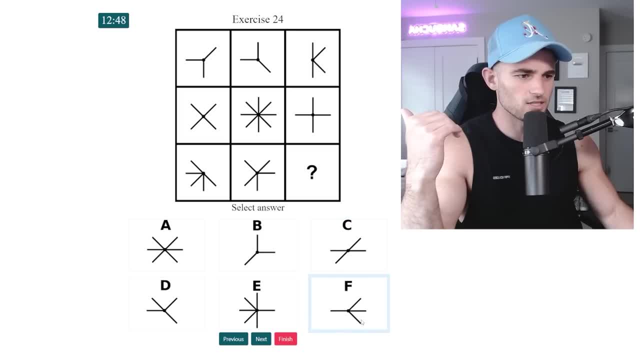 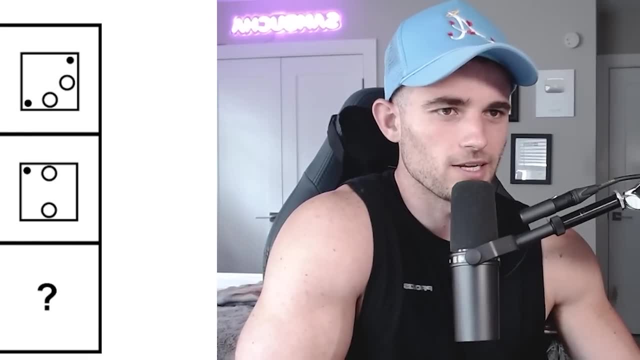 that looks good. no, but we have to eliminate that. so it could be this and it is this, so we're going to eliminate this. i'm pretty positive. it's this f. all right, exercise 25. hopefully this is the last one. why would they give me more than 25 questions? i'm already like dead. okay, two, three, two, four, two. 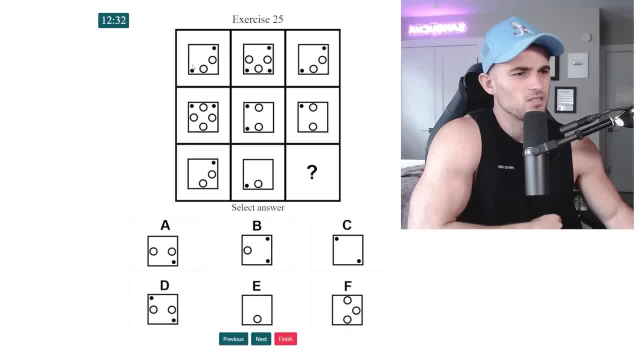 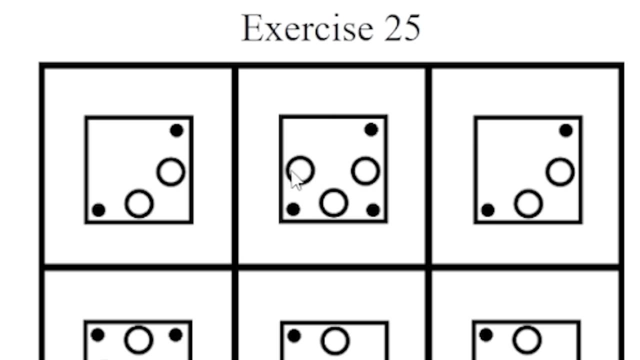 two. okay, so we can't do anything? additive- what about these dogs here? um, what is going on here? wait, why am i? this is? this is seeming pretty difficult now. so it's additive and removing what's not common, so in this case these are adding together. there's no middle left on here, and so 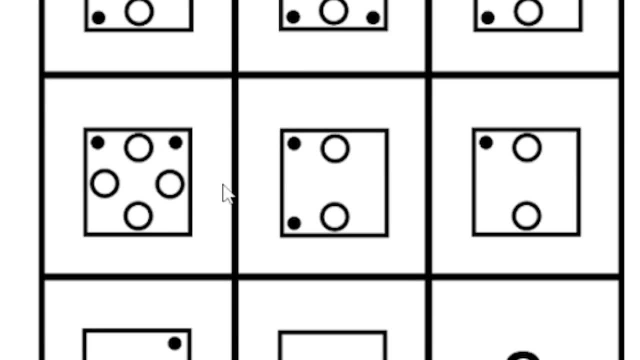 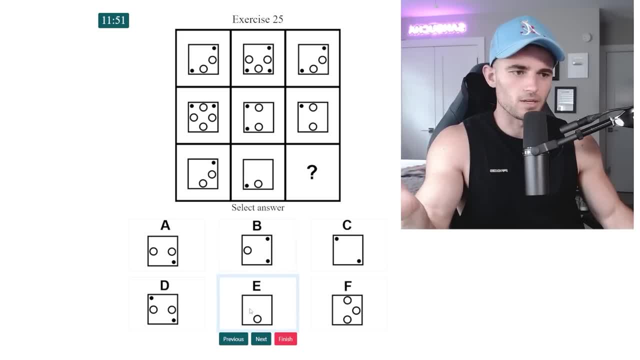 they're eliminating in here. so this is going to be two on top: eliminate there. this is going to be eliminating the dots. so there's going to be no dots and we're only going to retain the bottom gotta be. there's no common black dot and the only commonality is the bottom center. so e uh. 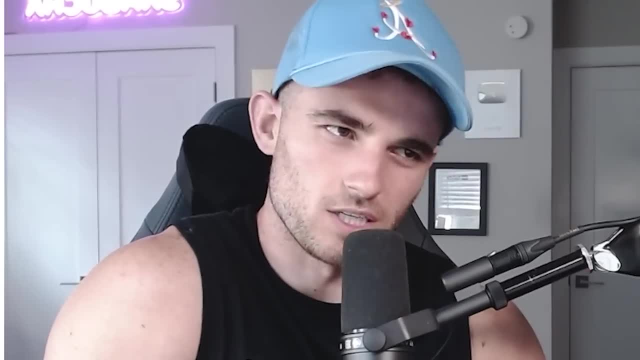 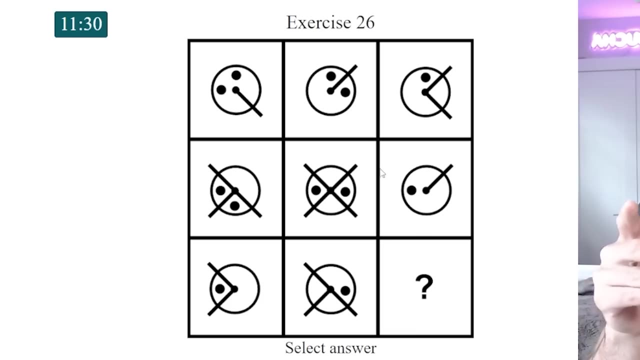 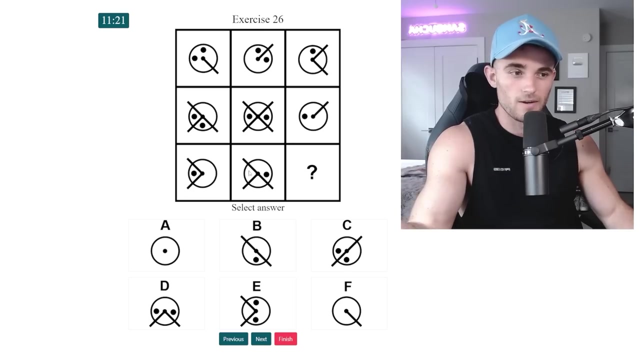 same idea here, so retaining this interesting. this is interesting. the circles are retained if they're common, but the lines need to be uncommon in order to be retained, so the circles need to be common. so in this case, for instance, the circles aren't common, there's going to be no circles, and then the lines are. 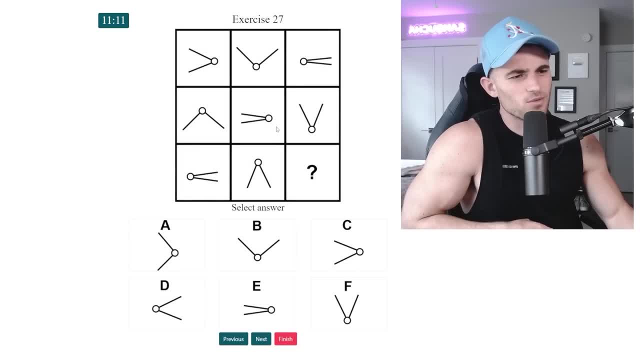 eliminated, so it's got to be f. yeah, there's no commonality, so we're looking like there's angles or something that we're going to be dealing with here. i don't have like a great idea of what this could be. i think it's going to be a wider one, just because there's a wide, a narrow and a standard one. 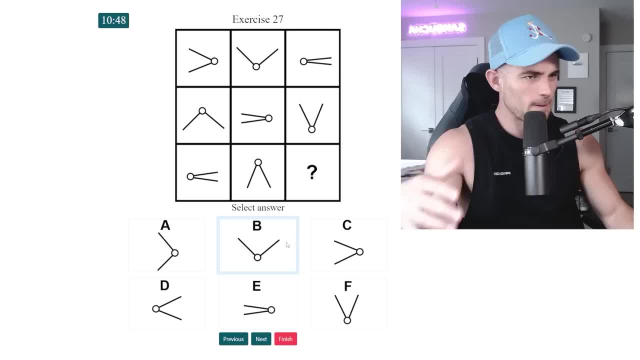 so it's going to be something wide, so it's going to be a or b in terms of direction, it's hard to say like. so it's not going to be a flip-flop. so what's going on here? so you have a circle pointing right, left and down. all right, this one, i don't think i'm going to have a lot of certainty. it. 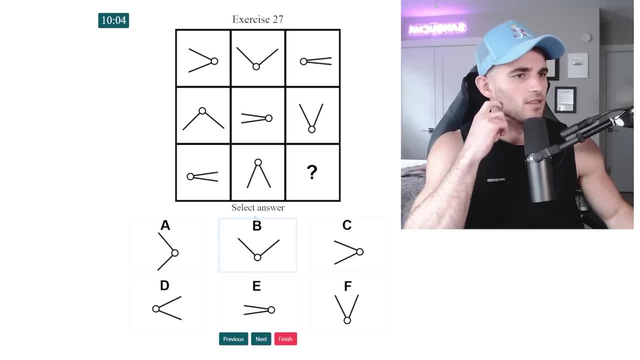 might just be like something random. so far, i mean so far, they've only gone up or down. so do we break that mold? like it's clear that they're willing to repeat patterns, but it's not clear if they're able to kind of flip over the axis, although the standard one 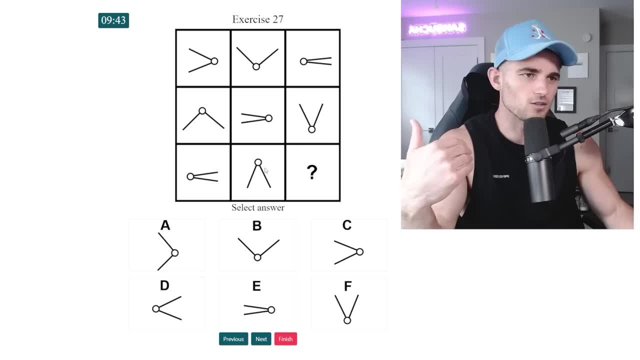 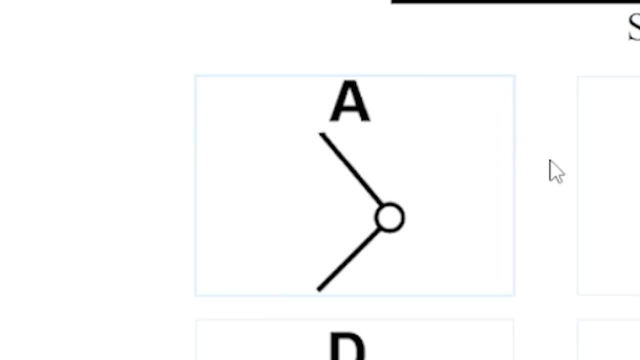 does, because it's horizontally facing, and then it goes vertically facing and then it goes back to this, this, this, this. this is what's throwing me off these middle ones. oh okay, bam, bam, bam, it's gonna be a, because it's it's clock, uh, clockwise rotating the opening of the angle. so it's got. 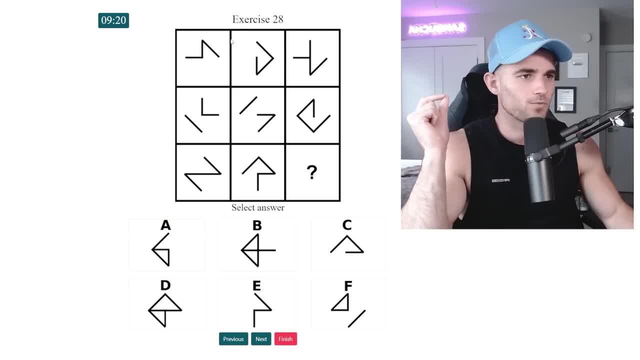 to be a. that took me far too long. okay, this is commonality. delete the commonality. so combine and delete the commonality. it looks like. let me just confirm. yep, it is okay. uh, so the commonality here is going to be this. so that's gone. so we're going to retain. 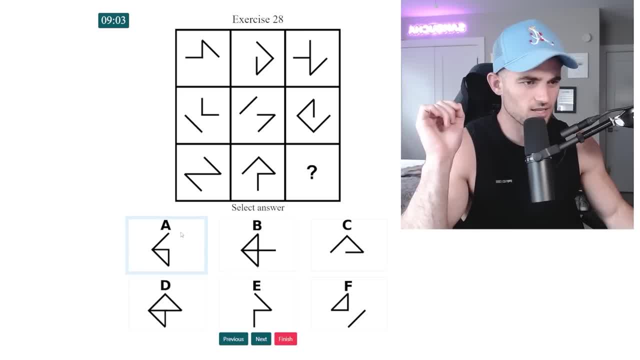 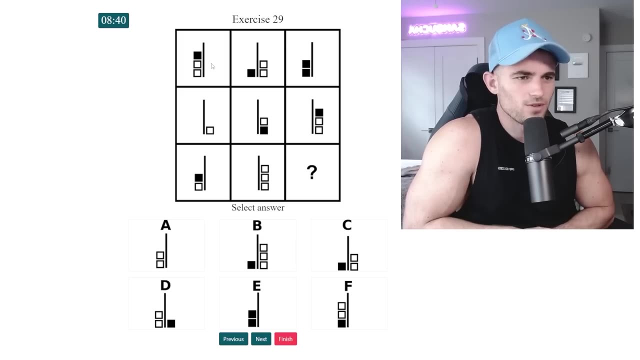 this, this, this, delete this. it's a. let me just make sure, hold on, hold on. just that one side is going to be gone. delete the commonality. right, that's the theme. okay, it's got to be a. so what is happening here? what are they alternating the? no, they're not. there's no alternating of the. 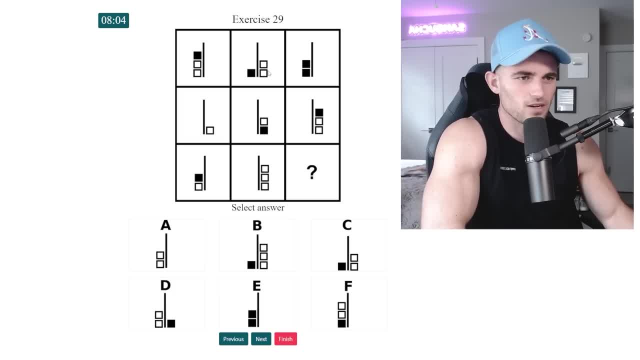 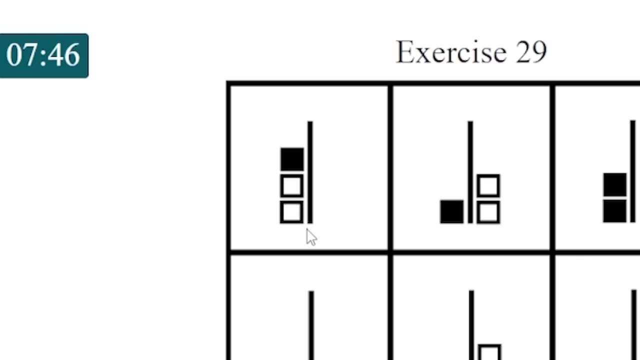 whites, not a commonality thing. is there like a flipping of the colors when you come? what? so? this plus this, so we have, oh, okay, okay, okay, wait, wait, wait. this makes sense. okay, i see, i see it's like think of it like: uh, this is like an equal sign. so this and this eliminate each other. 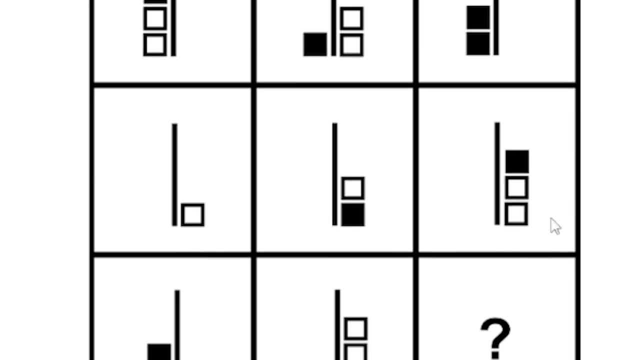 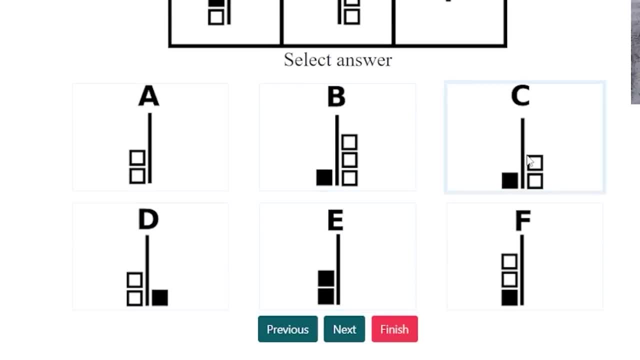 and then it's just these two left, so in this case they're on the same side, so everything's retained. so in this case there's going to be two on the right and the black is retained on the left, so it's going to be c. does that make sense? so there's three here. there's one on the left side. on this: 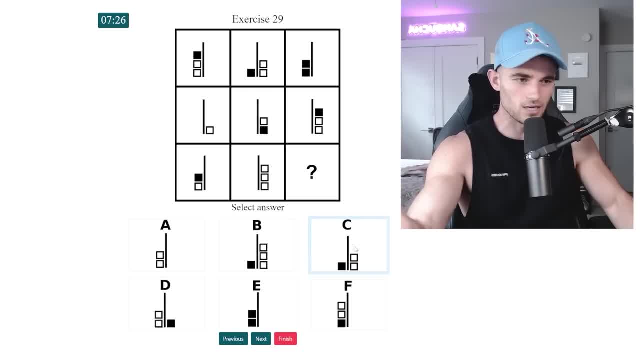 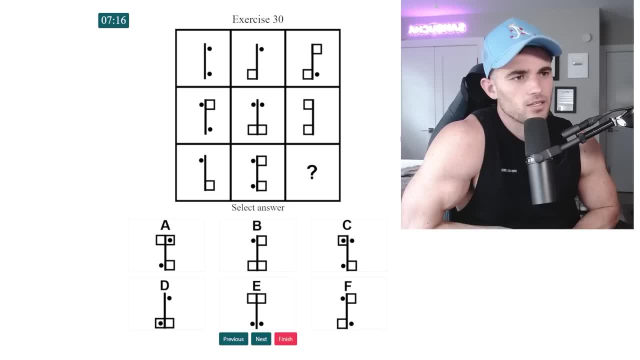 pattern, so it's going to be two. that's left on the right. there's no block competing with it, so it's going to be c. okay, please be the last one. i'm like kind of mentally done after this. uh, all right, let's see. is it the same idea? so it's going to be circles up top, aren't there? because they're common. 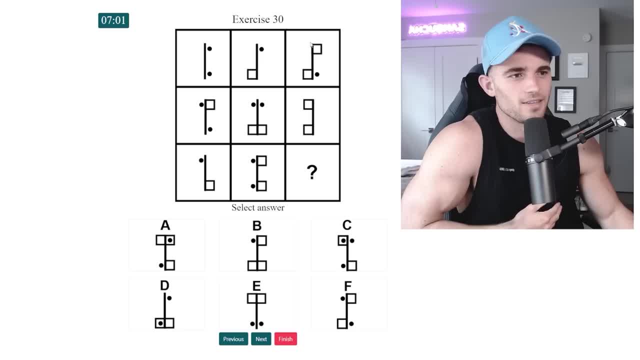 so that could be it, but then again probably not, because why is then this here? like how does this square come to play? like i don't know what happens. something happens, i don't know what's going on. like why is there zero dots here? i have to figure that out as well. let's solve for the dot first, because we know that. 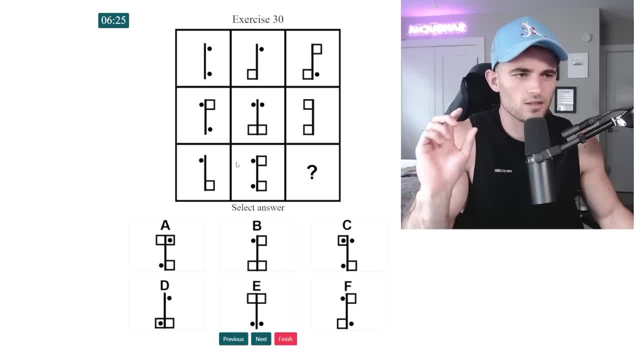 this is the same as this, just the left side. the dots are on the left side, effectively, so we can assume there's going to be a black dot in the top left. so i so far i say b, c or f, just based on that alone, and then if we're going off of, there's just not that much data to go on. 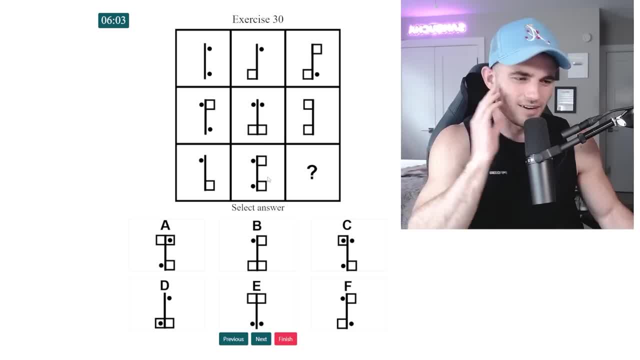 and then if we're going off of, there's just not that much data to go on because we don't have anything similar to this, so i don't even know what's going on with this. so if they're all same side, i don't know. i think this is the one. we just go raw. i'm. 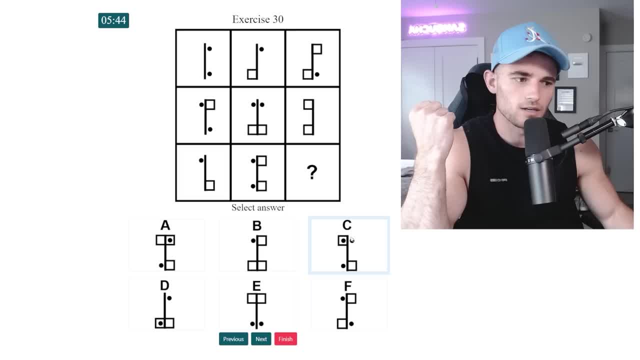 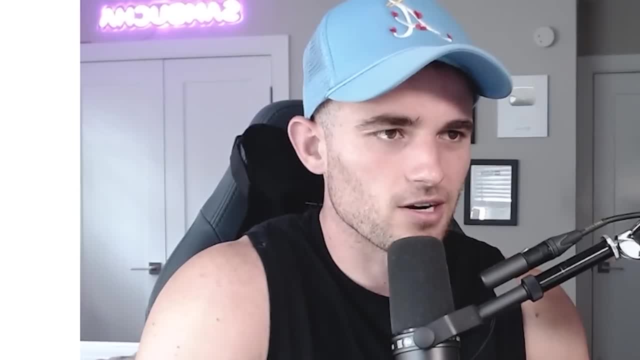 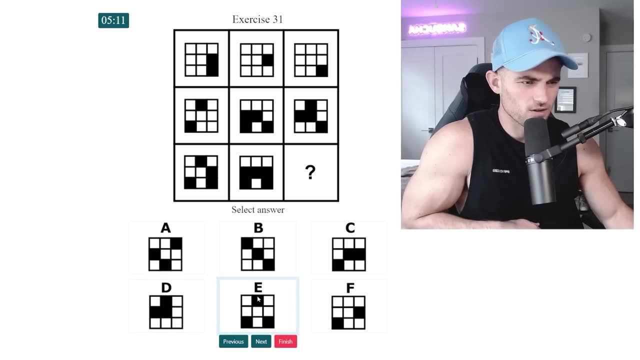 gonna go with. i think we just go b, because there's only one dot. i know that's dumb logic, but another one. okay, all right, all right, all right, this is easy enough. this is just delete commonalities. again, this is highlighted up top, so it's drf good, and then gotta be deep. yeah, because this eliminate. 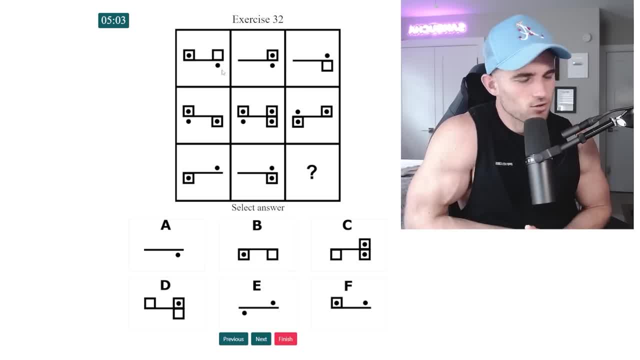 yeah d okay, bam, keep going. the dots are throwing me off big time. i'm not gonna lie to you guys. this is really taking a toll on me. so everything's eliminated. like what happens? that it flips. i don't get it. like what is happening, that this needs to flip. it looks like there's an agreement that. 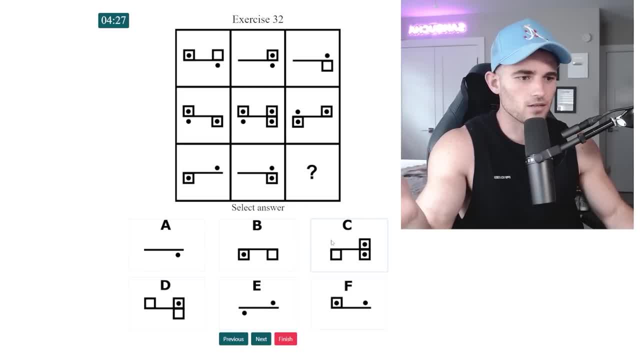 the dot is going to be in the top right, just based on backs. so i think it's going to be d, e, f or c- the amount of available squares, i don't know what that's going to be. it might be three, because that's common. i mean, this is like really kind of dumb trial and error i'm doing, but it feels like. 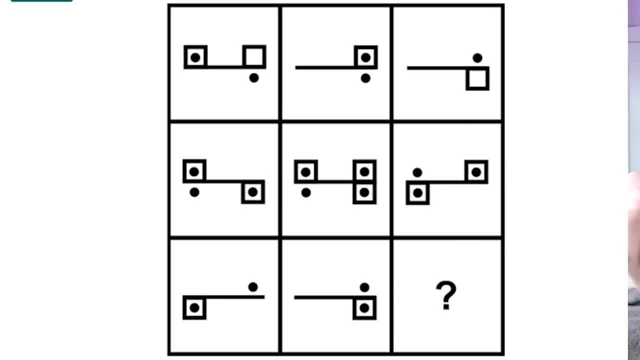 d is the right answer, because the dots aren't going to be retained. something's going to happen to them, as evidenced here and here. like you, never have the two side dots retained, so after that you can't expect this. so i think d is the most reasonable. i guess. yeah, i don't know, i guess.